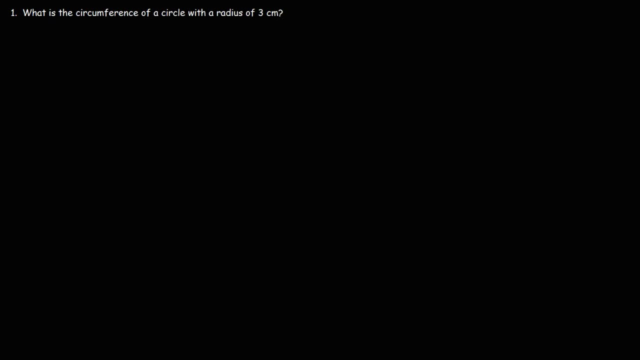 In this video we're going to talk about how to calculate the circumference of a circle. In this example, we're given the radius of the circle, but let's draw a picture. The radius is the distance between the center of the circle and any point on a circle, and in this example that's three centimeters. Now what is the? 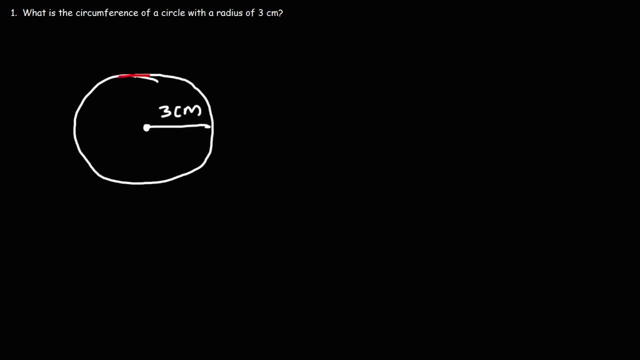 circumference of the circle. The circumference of the circle is basically the distance around the circle. You could think of it as the perimeter of the circle, and there's a formula that we could use to calculate the circumference. It's C is equal to 2 pi times R, where R being the radius of the circle and all. 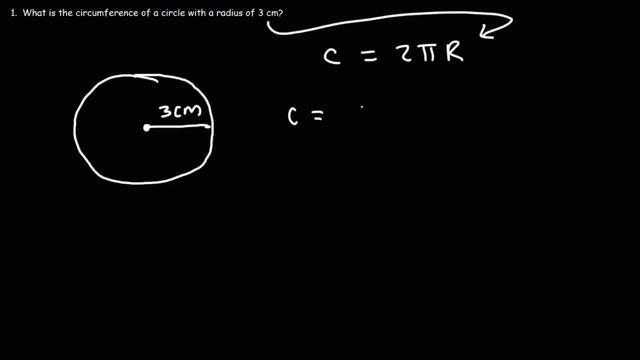 we need to do is plug in R into this formula and we're going to get the answer. So it's 2 times pi, and for pi I'm going to use the value three point one, four one, five, nine times the radius of the circle, which is three centimeters. 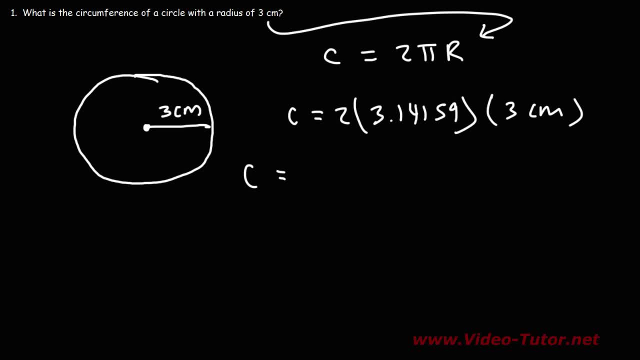 So two times three point one, four, one, five. nine times three, That's 18.85 if you round it approximately. Now, what are the units of circumference? The units for the circumference of a circle will be the same as the unit of the radius of the circle. In this case it's going to be centimeters. So this is the answer. 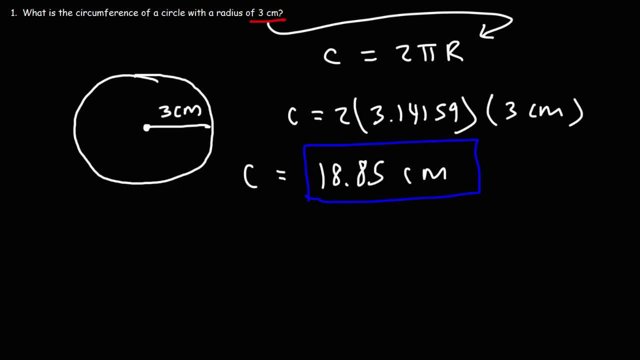 to the problem. The circumference of this particular circle is approximately 18.85 centimeters, and I should use the approximate symbol, since this is a rounded answer. Now let's move on to the second problem. What is the circumference of a circle with a diameter of? 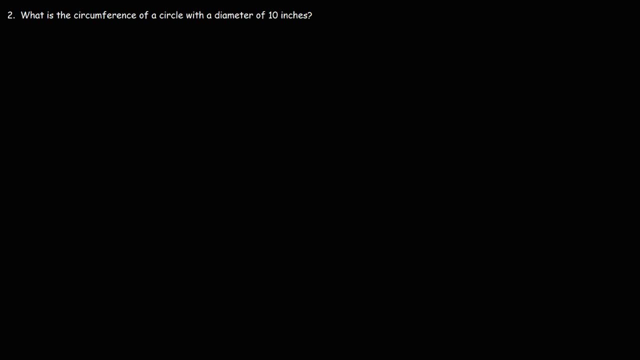 10 inches. So let's draw a picture. The diameter of the circle is basically a line that starts from one end of the circle and passes to the other end, but it goes through the center of the circle. So that is the diameter of the circle. Now, what you need to know is that the diameter 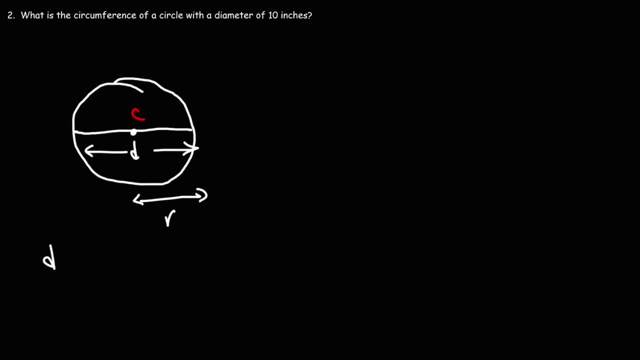 is twice the value of the radius of the circle, So d is equal to 2r. Thus, to get the radius of the circle you need to divide the diameter by 2 or multiply by half. So if the diameter is 10 inches, the radius of the circle is going to be half of that. 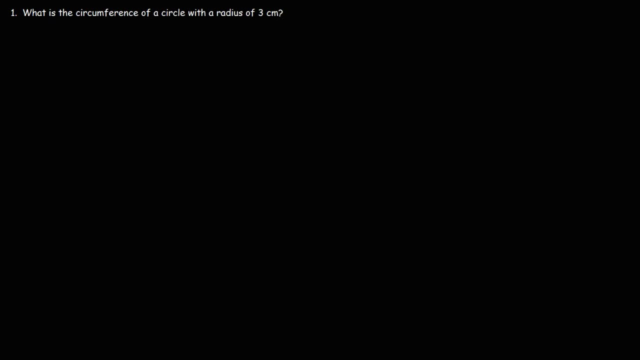 In this video we're going to talk about how to calculate the circumference of a circle. In this example, we're given the radius of the circle, but let's draw a picture. The radius is the distance between the center of the circle and any point on a circle, and in this example that's three centimeters. Now what is the? 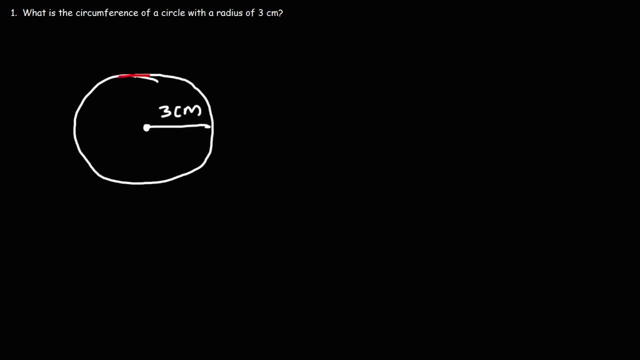 circumference of the circle. The circumference of the circle is basically the distance around the circle. You could think of it as the perimeter of the circle, and there's a formula that we could use to calculate the circumference. It's C is equal to 2 pi times R, where R being the radius of the circle and all. 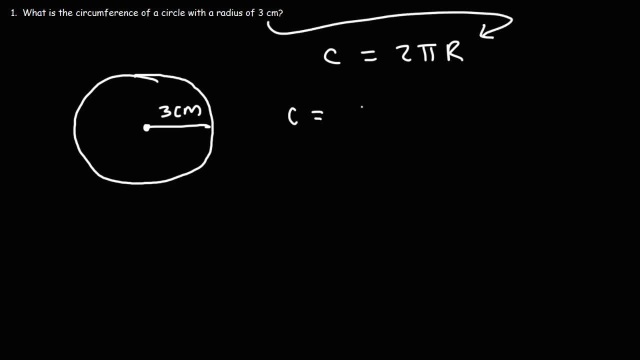 we need to do is plug in R into this formula and we're going to get the answer. So it's 2 times pi, and for pi I'm going to use the value 3.14159 times the radius of the circle, which is three centimeters. 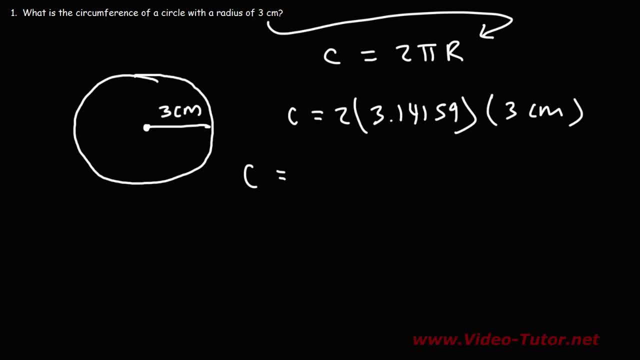 So 2 times 3.14159, times 3,, that's 18.85 if you round it approximately. Now, what are the units of circumference? The units for the circumference of a circle will be the same as the unit of the radius of the circle. In this case it's going to be centimeters. So this is. 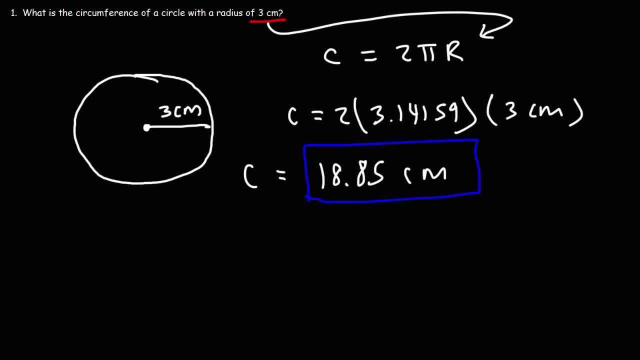 the answer to the problem. The circumference of this particular circle is approximately 18.85 centimeters, and I should use the approximate symbol, since this is a rounded answer. Now let's move on to the second problem: What is the circumference of a circle with a diameter of 10 inches? 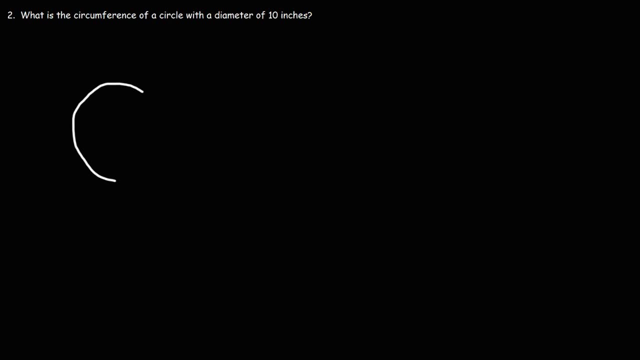 So let's draw a picture. The diameter of the circle is basically a line that starts from one end of the circle and passes to the other end, but it goes through the center of the circle. So that is the diameter of the circle. Now, what you need to know is that the 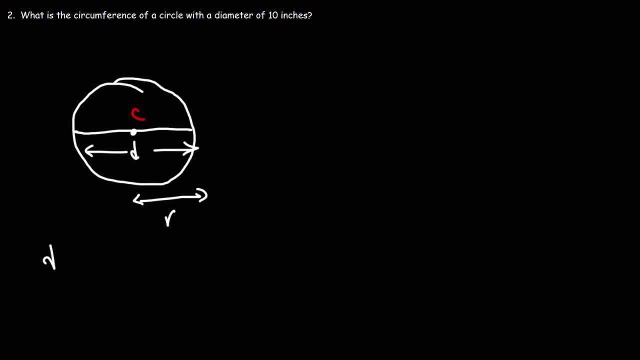 diameter is twice the value of the radius of the circle, So d is equal to 2r. Thus to get the radius of the circle you need divide the diameter by 2 or multiply by half. So if the diameter is 10 inches, the 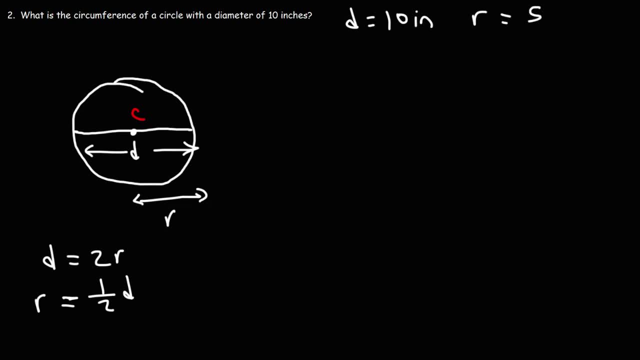 radius of the circle is going to be half of that. Half of 10 is 5.. Now, once we have the radius of the circle, we can now calculate the circumference using the same formula that we used in the last problem. So it's going to be 2 times pi. 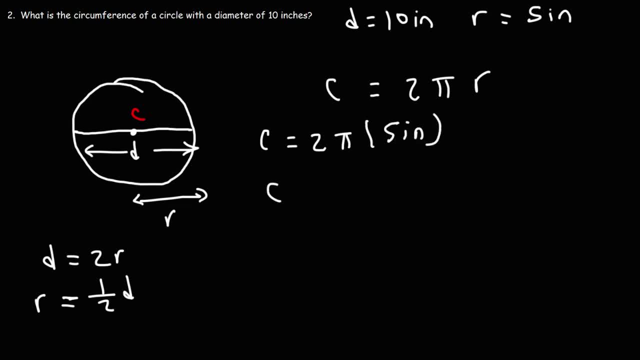 times 5 inches. So 2 times 5 is 10, thus the exact value for the circumference of the circle is 10 pi inches. But if you want to turn that into a decimal value, we can say that C is approximately 10 times 3.14159.. So we can round that to. 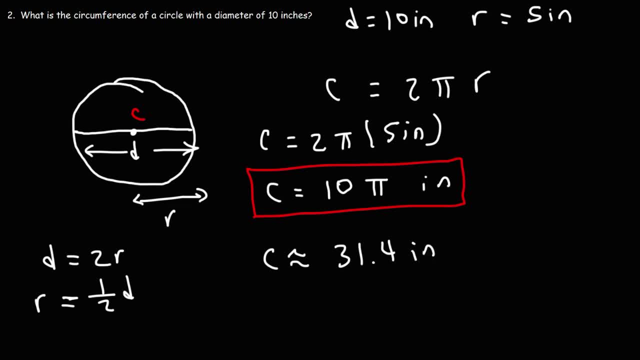 31.4 inches. So that's how you can calculate the circumference of a circle, given the diameter. You just need to find the radius first, and then you could use this formula to get the answer. Now let's move on to the last question of this video. 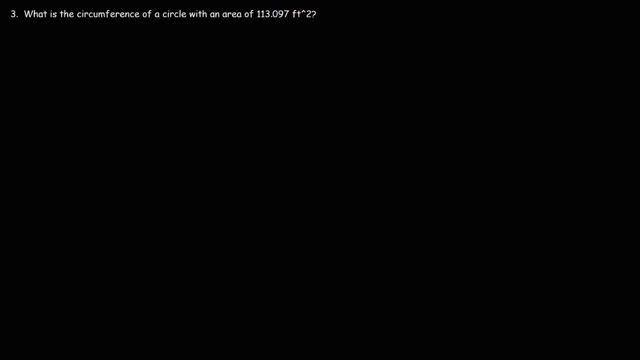 What is the circumference of a circle with an area of 113.097 square feet? Well, the area of a circle is pi r squared. We could use this formula to calculate the radius of the circle And then, once we have the radius of the circle, we can calculate the 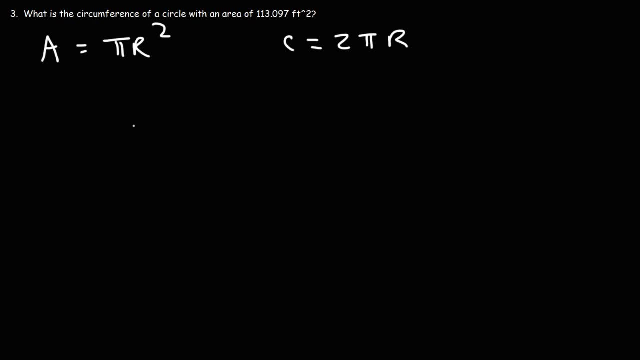 circumference using the formula on the right. So let's calculate the radius. So the area is 113.097, and that's going to equal pi times r squared, And for pi we're going to use 3.14159.. So first we're going to divide both sides by pi. 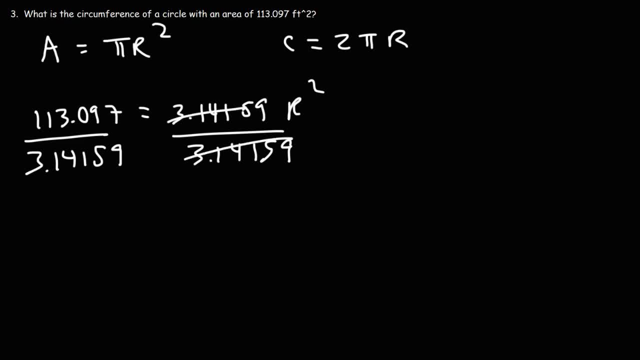 113.097 divided by 3.14159.. That's 35.9999, which is basically about 36.. And now we can take the square root of both sides. The square root of 36 is 6.. So the radius is approximately 6 feet. 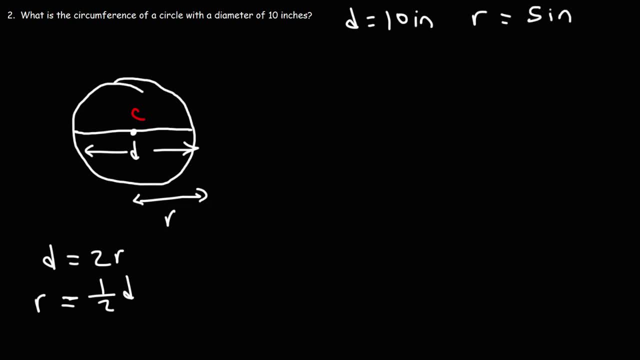 Half of 10 is 5.. Now, once we have the radius of the circle, we can now calculate the circumference using the same formula that we used in the last problem. So it's going to be 2 times pi, times 5.- 5 inches. So 2 times 5 is 10.. Thus, the exact value for the circumference of the circle is 10 pi. 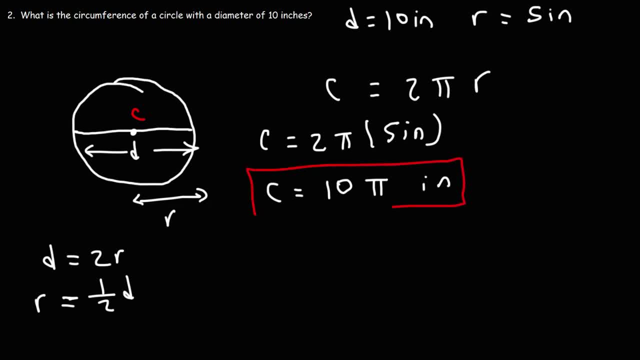 inches. But if you want to turn that into a decimal value, we can say that c is approximately 10 times 3.14159.. So we can round that to 31.4 inches. So that's how you can calculate the circumference of a circle. 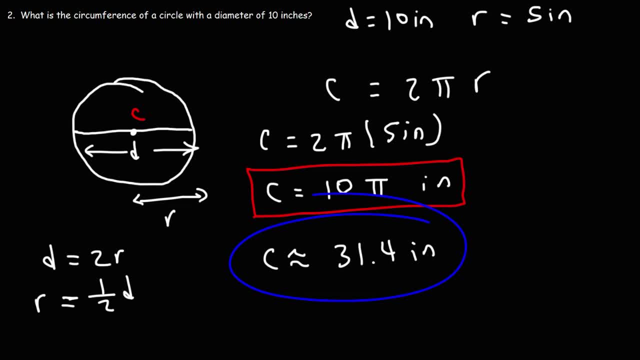 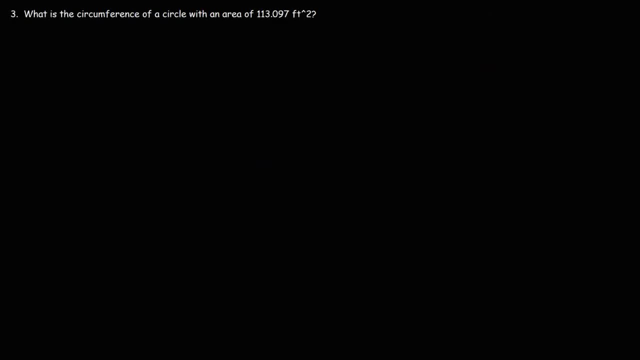 Now let's move on to the last question of this video. What is the circumference of a circle with an area of 113.097 square feet? Well, the area of a circle is pi r squared. We could use this formula to calculate the radius of the circle And then, once we have the radius of the circle, we can. 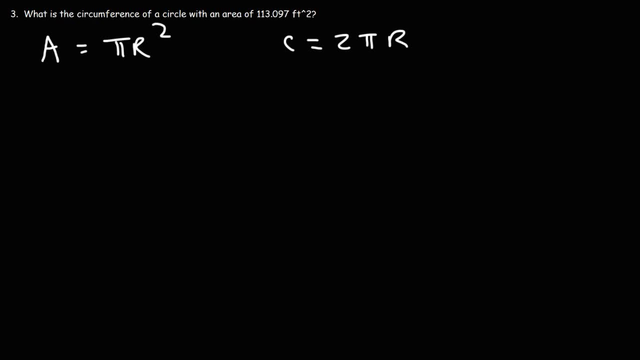 calculate the circumference using the formula on the right. So let's calculate the radius. So the area is 113.097 and that's going to equal pi times r squared, And for pi we're going to use 3.14159.. So first we're going to divide both sides by pi. 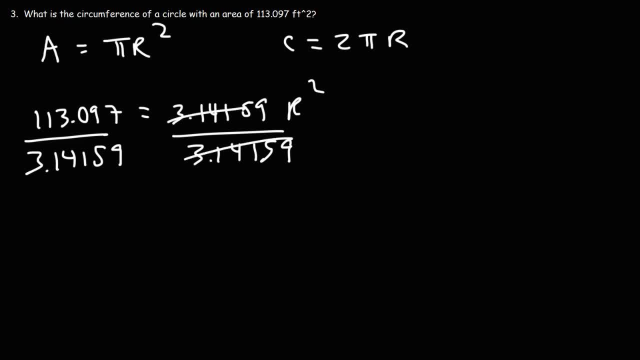 113.097 divided by 3.14159.. That's 35.9999, which is basically about 36.. And now we can take the square root of both sides. The square root of 36 is 6.. So the radius is approximately 6 feet. 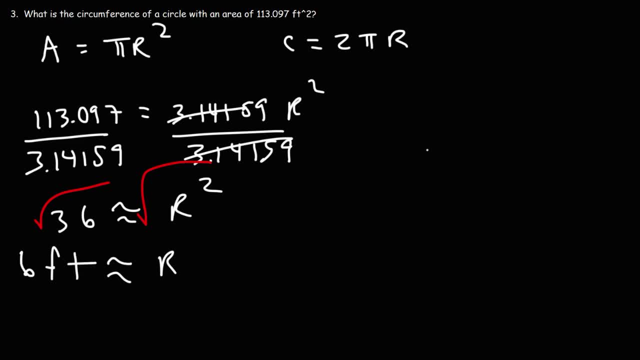 So now we can take that and plug it in to that equation. So c is going to be 2 pi times 6 feet. So the circumference is approximately 12 pi feet. So multiplying 12 by 3.14159 we can say that the